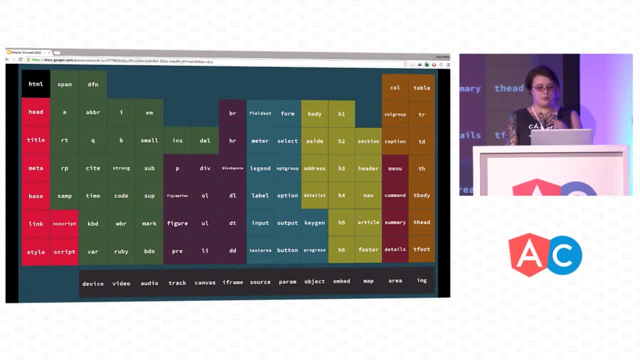 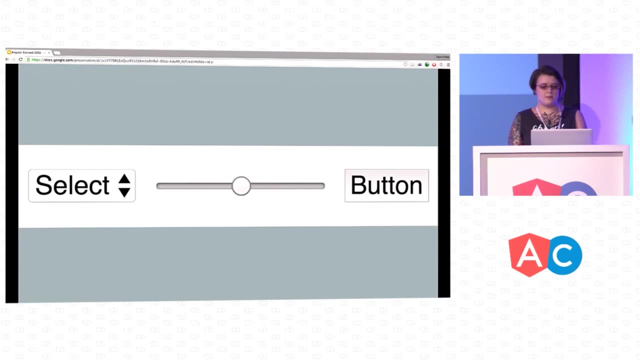 Custom elements are important to this. In a sense, elements are the only way we're able to provide a graphical user interface on the web. This is true even for WebGL, which employs the canvas element. Many standardized elements represent GUIs. So when we implement web UI components, making them elements is. 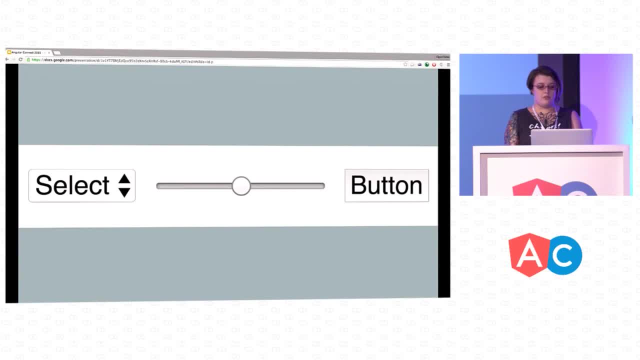 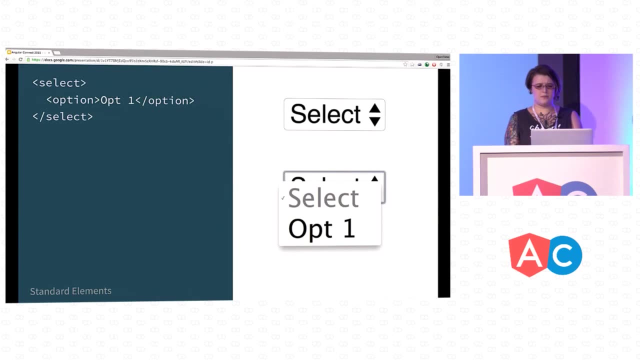 frequently the best choice, Because the result will have the advantages of familiarity and flexibility within the context of the web platform. Corkiness is not an admirable trait in an API, Since Angular 1 directives imply that we could already make custom elements. what's so special? 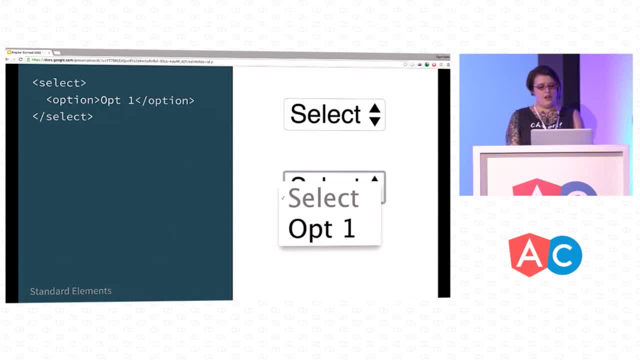 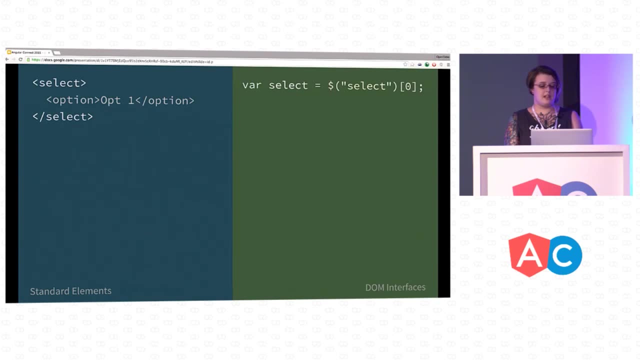 about an official custom elements specification. It's in how a nonstandard element is different from a standard element. When the browser parses mark up into a DOM document, tags that are recognized by the browser get special treatment. For example, take a standards-like. 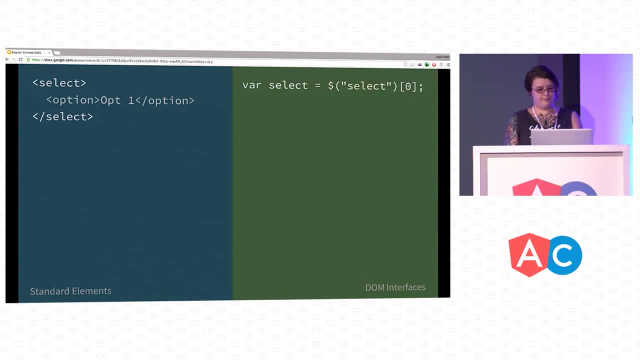 We can access properties and methods that are specific to SELECT. One such specific property is the options property. This is a collection of all the options of the SELECT which we can examine and manipulate. The SELECT element also has an add method. The add method allows us to imperatively add a new option to the SELECT. 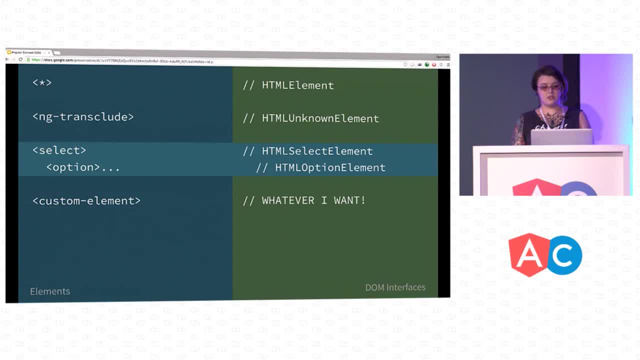 A SELECT has its hand-tailored interface defined in the DOM specification. nonstandard and therefore unrecognized elements are only able to have the interface of HTML unknown element which is totally identical to the bare bones HTML element interface. The custom element specification will allow us to make custom elements that the browser 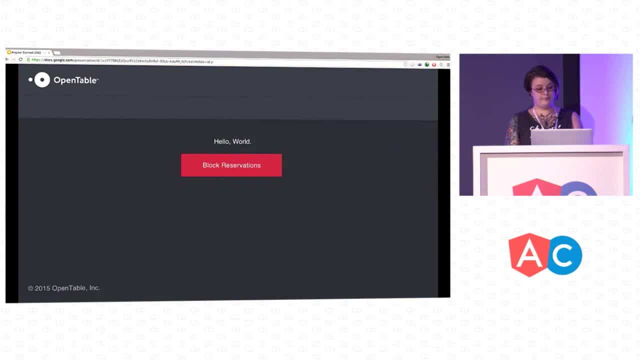 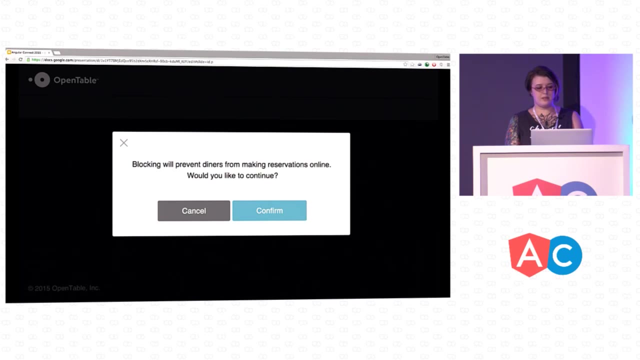 can bootstrap with custom interfaces that we define. In order to explore programmatic interfaces, we'll implement an example modeled on a product enhancement that we recently developed at OpenTable. Certain existing restaurant operations features need a confirmation. Instead of immediately proceeding, we ask the restaurateur to confirm. 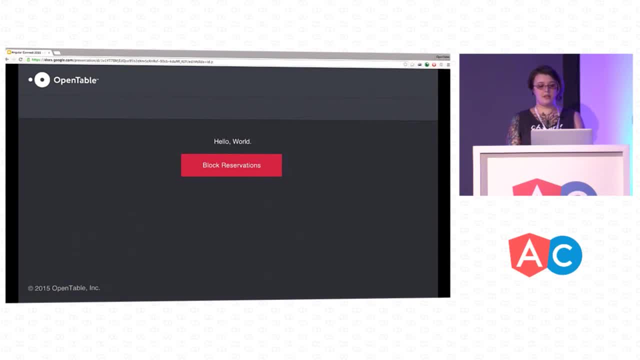 By implementing the confirmation as a component, we enable application developers to add the entire confirmation workflow on top of a feature like this one with minimum disruption to the feature's existing code. but how successful we are at that depends very much on the programmatic interface that we choose. 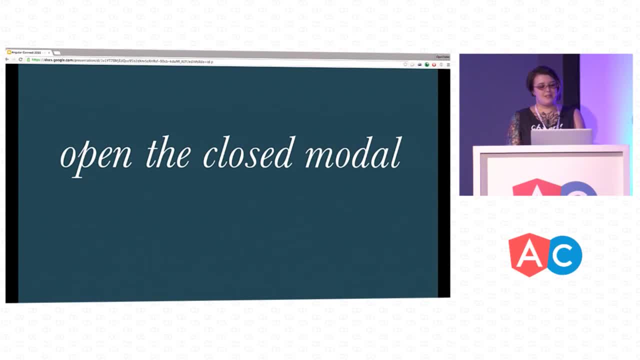 So how will we choose it? Well, being able to add methods and properties- Most elements- allows us to utilize some classic advice. Take a simple, plain English statement of what we're trying to accomplish, such as: open the closed modal. Not surprisingly, the noun is the modal. 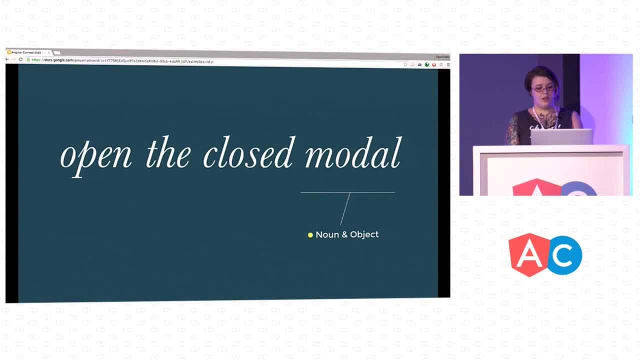 That becomes our object and therefore our element. Qualities that the modal may have like- is it currently open- are properties on the object reflecting adjectives and the functionality of the element can be expressed as methods on the object for verbs like the open action. 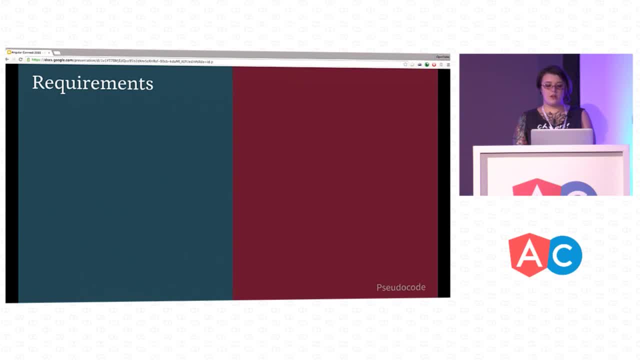 Just as user experience design does from the perspective of the user, we can design our API primarily from the perspective of the application developer by focusing on the functionality the UI component must provide, rather than how to provide it. First, the application developer needs a way to request confirmation. 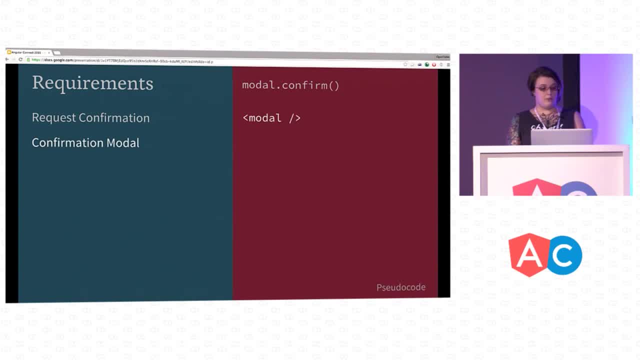 Confirming is an action Which means confirm should ideally be a method on the modal, and the application developer needs a way to request confirmation. confirming is an action which means confirm should ideally be a method on the modal, And after the application has requested confirmation, the modal dialogue must appear. 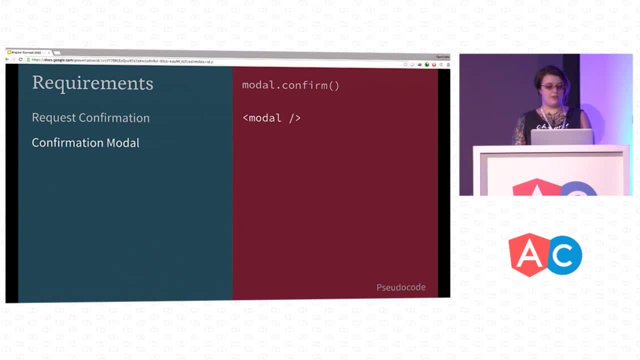 The fact that the modal is the GUI that the customer will see, the part that has visible presence on the page- is another reason the modal itself should be the custom element. The modal can appear because the modal opens. Opens is an action, which means it's another method. 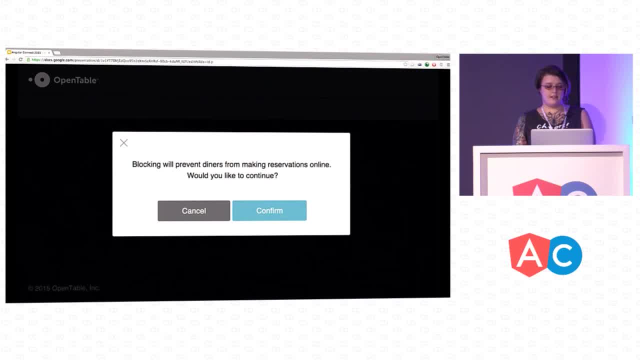 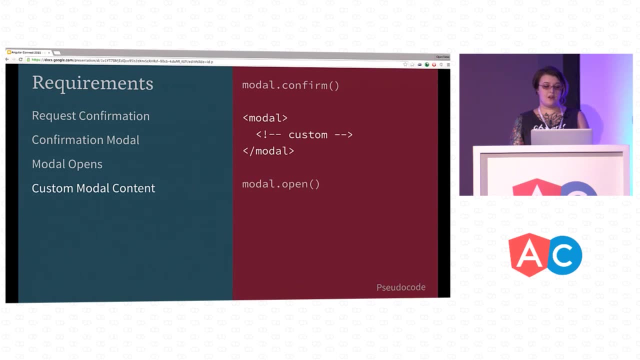 Let's examine the open modal. There's content inside, some of which we'll build in. However, this example with two buttons shows that the advisory information in the modal may be different for each specific feature, So the application developer needs to be able to customize some of the content in the confirmation. 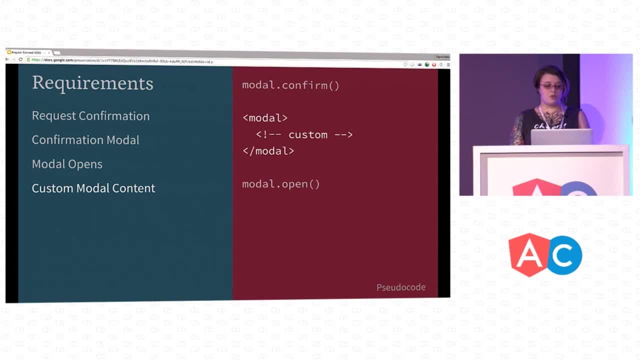 modal. Since this will render like typical marked-up text, we'll treat the modal like any standard container and allow nested HTML. Protecting several features means we might want to have multiple modals at a time. It must be possible to do so. 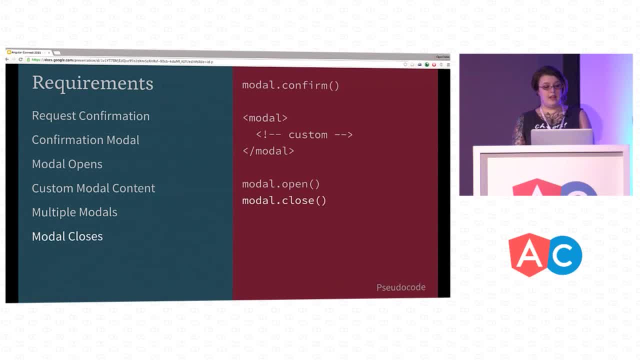 And to associate- We're using the correct modal- with the feature. Next, after the customer has confirmed, the modal needs to get out of the way so that the customer can continue working. consequently, the modal needs to close. Another action, another method. 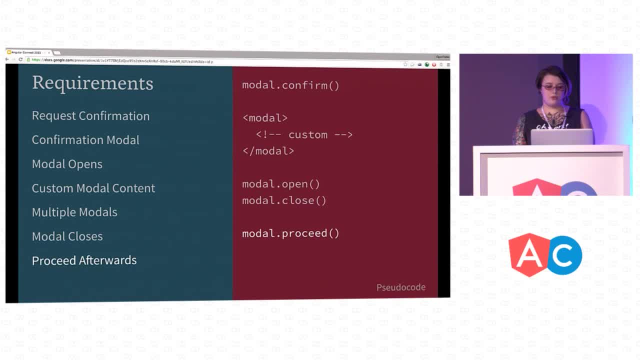 Then we want to continue using the application's original code to block reservations. So the next to the last requirement is that there must be a way to proceed with the original functionality. There are a number of options for how to enable it. It may be correct and incorrect. 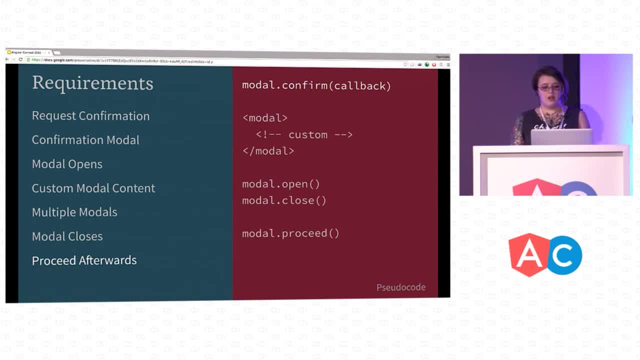 OK, And so that's the first and last step we're going to take. Next is the final step. We'll take a second. Next, to enable the reuse of the application's original code, we'll have the application provide a callback. 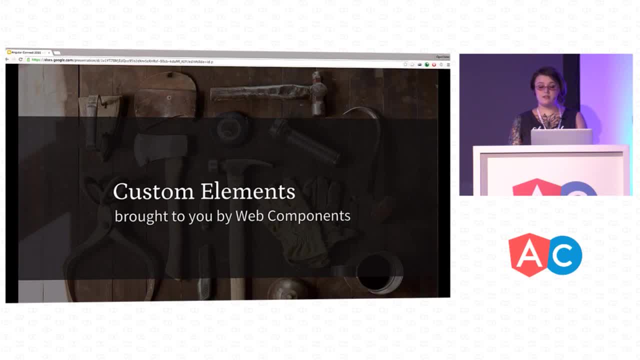 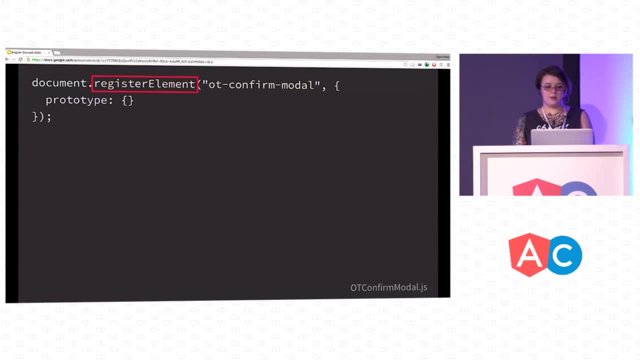 Now that we have our requirements, let's try building our confirmation modal as a custom element. To start, we use a new method from the custom element specification, registerElement, to register the element with the browser. The first argument is the type or the custom element's tag. 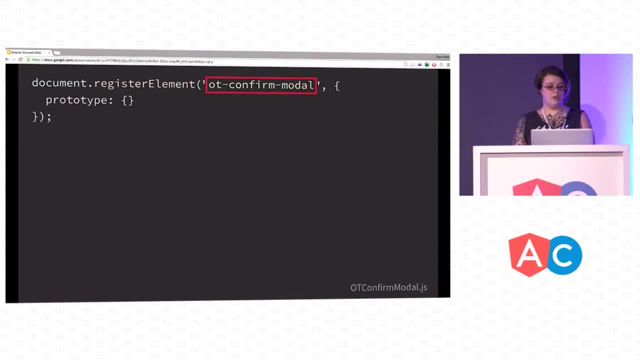 name. We'll register our custom element as otConfirmModal with a hyphen. A custom element has to have a hyphen in its type. The second argument configures the custom element. Defining the prototype property with an object allows us to provide the custom interface that we just planned. 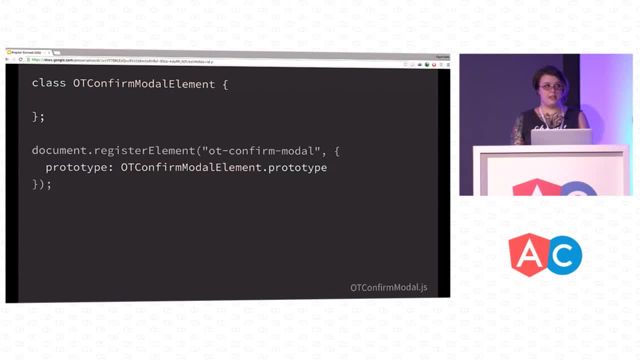 When it comes to creating the prototype object, there are lots of options. Any way of creating an option will do, I like using an ES6 class and its resulting prototype. Just like standard elements, we can create a custom element from the HTML element interface. 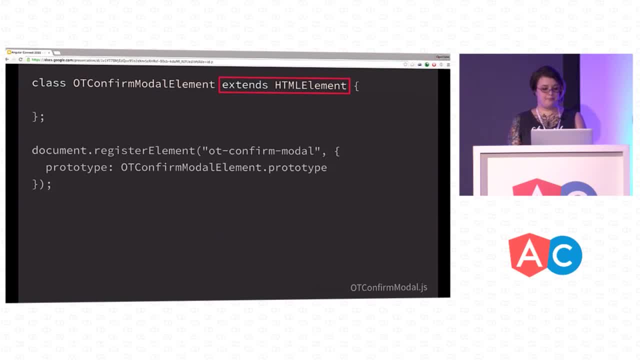 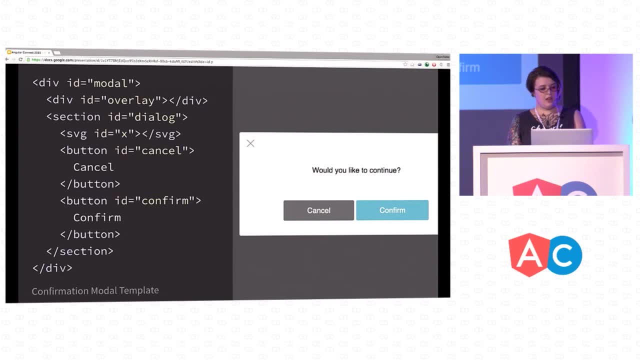 Adding the extends keyword to our class signature sets that up. Now let's make that built-in GUI- Assuming that we have already readied a template for the modal, with the overlay, the dialog, the close icon, one cancel button and one confirm button. 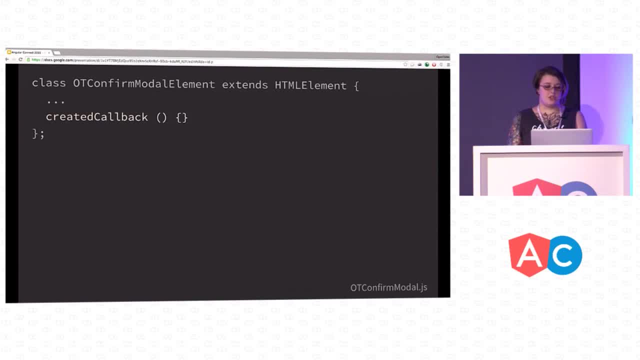 The custom element specification also defines several life cycle callbacks for important milestones in the element's life. Created callback is the earliest point, making it the ideal place to add our template. I'm not going to go into specifics about this, since we focused on that in our content. container components. 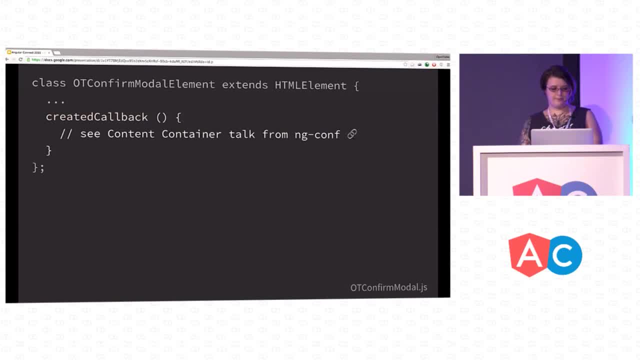 talk at ng-conf and we'll link that from these slides. In addition to life cycle callbacks, we can add open and close methods. These will become visible to the application developer in the DOM. An interesting way to implement opening and closing the modal is to use the hidden property. 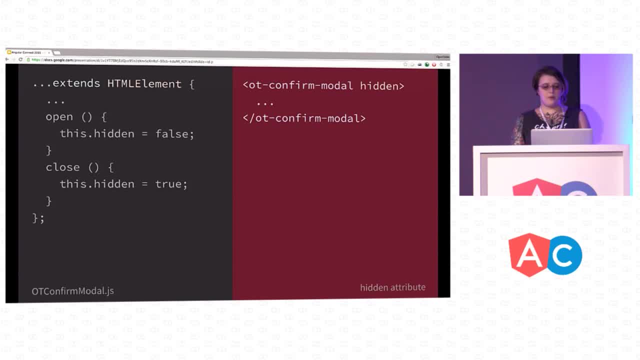 Hidden is interesting because it's a pre-existing HTML element property that will be automatically reflected to the element's attributes. This illustrates a noteworthy fact. By default, custom properties are not automatically published as attributes. This means having a fully declarative option with attributes. requires some extra work. 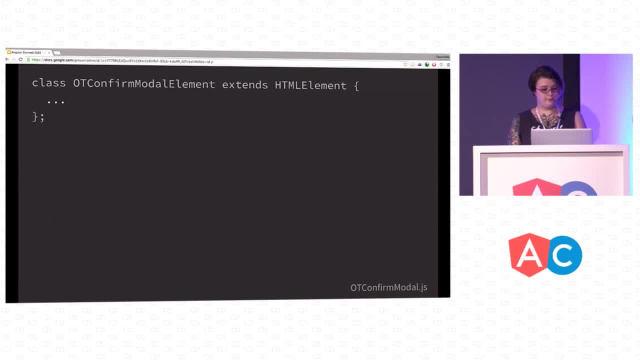 and that's one of the advantages to using Angular 2.. The last remaining requirements are requesting confirmation and proceeding afterwards. The confirm method is the primary entry point for the application to integrate the modal. Confirm saves the application's callback for later and opens the modal for the customer. 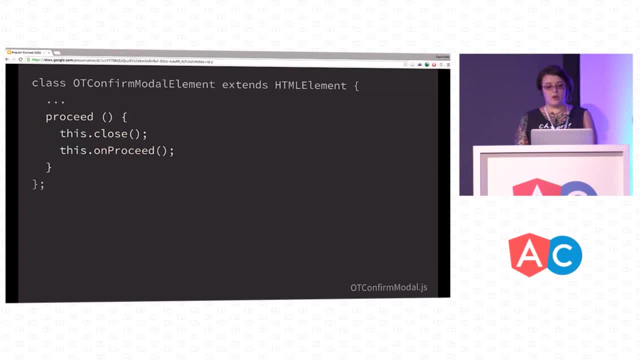 Finally, we define the proceed method that can be called when the customer clicks the confirmation button. Proceed closes the modal And runs the saved application callback. That's just a simple overview of this implementation. More detailed code and examples of additional options will be available soon in the GitHub. 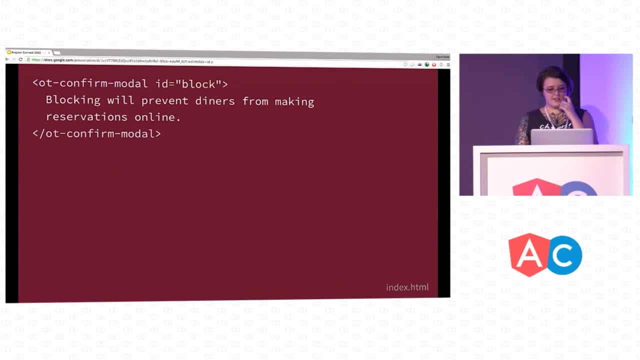 repo linked from the slides. So how does this look when an application uses the confirmation modal? First the application developer will add the OT confirm modal tag to their page with appropriate custom content. Then the application developer will query the DOM for the modal. 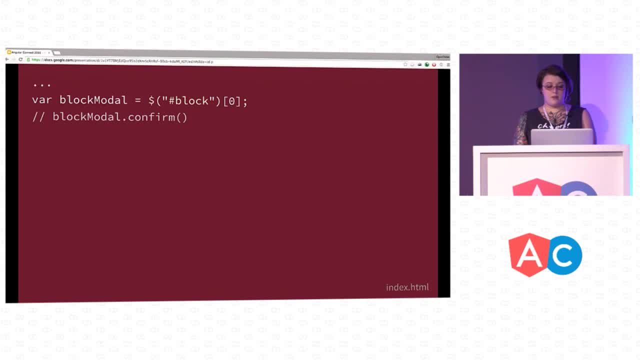 In order to be able to call its confirm method. Because the confirm method is on the element instance, calling confirm on the element with the ID block is completely unambiguous, which allows us to have multiple modals. Where and when to call the confirm modal depends on the application, of course. 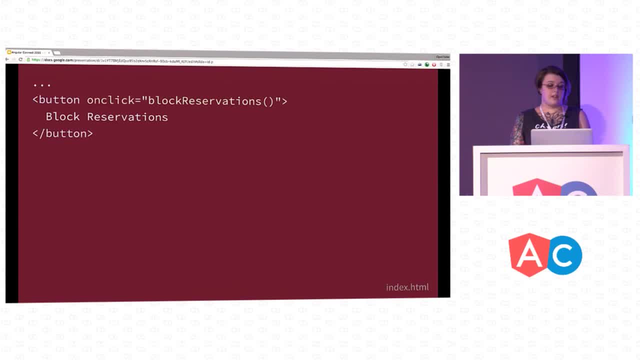 As an example that's somewhat similar to Angular. take the buttons on click attribute. The previous call to the original block reservation's functionality will be replaced with a call to the modal's confirm method And block reservations will be passed as a callback. A custom element is simple to use. 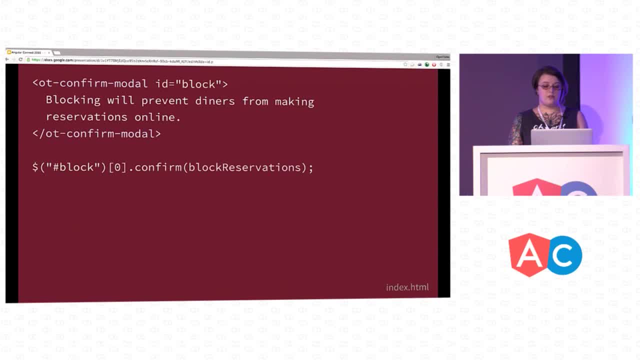 Minimally disruptive to existing code And makes our UI component feel very much like a standard element. And if we look at the programmatic interface, we can boil down to two main features. First, you can declaratively use the custom OT confirm modal tag in just the same way. 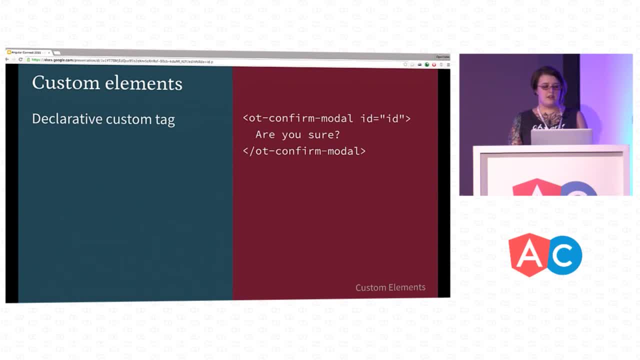 you might use a div. Besides facilitating custom content, this helps us annotate our markup And make it more readable. It allows at-a-glance understanding of what the code does. Second, you can imperatively access the elements public API from anywhere by querying the DOM. 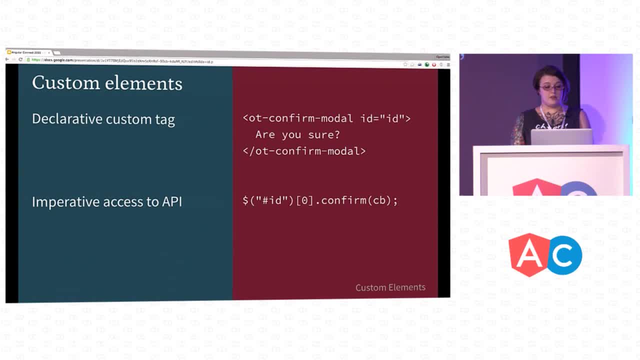 This is a powerful feature that not only makes the DOM more expressive, it also gives the developer a lot of flexibility in using the component. The application can decide when, where and how to call the component's methods. So, while in some ways, custom elements may not seem to be a major shift, 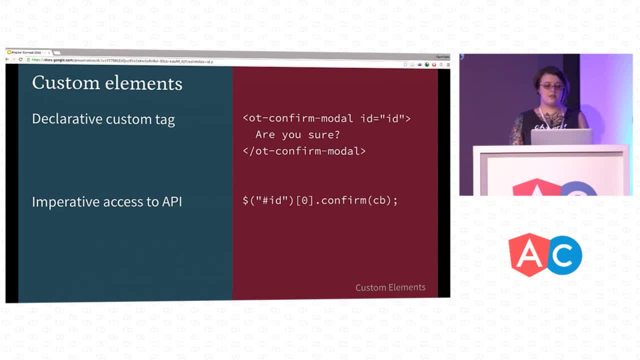 The impact of being able to extend the DOM is subtle, but very significant. Still, there are reasons why we utilize a full application framework like Angular, And benefits to doing so. Now I'll hand off to Kara, who will show us what we can accomplish with Angular. 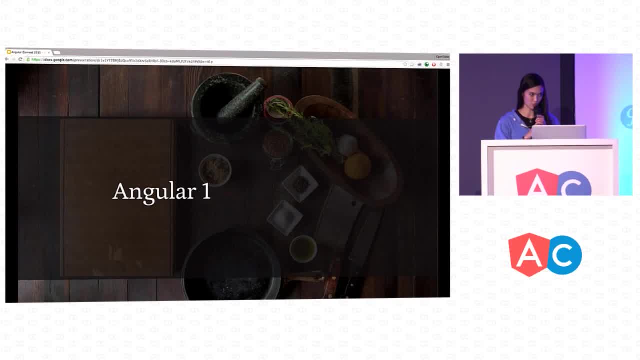 Hello, Oh, great, Okay, Okay. So, having reviewed the possibilities that custom elements permit, we've come to the conclusion that custom elements permit can be used in a lot of different ways. One of the things that we've found is that custom elements permit can be used in a lot. 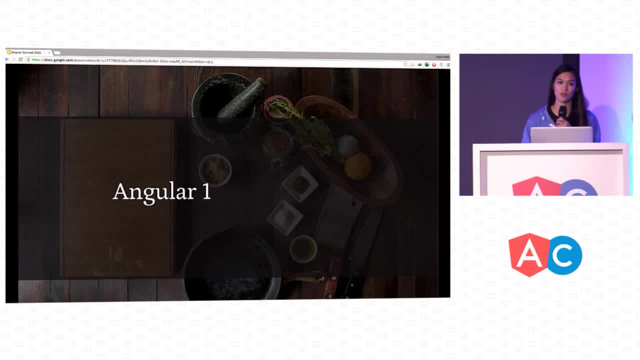 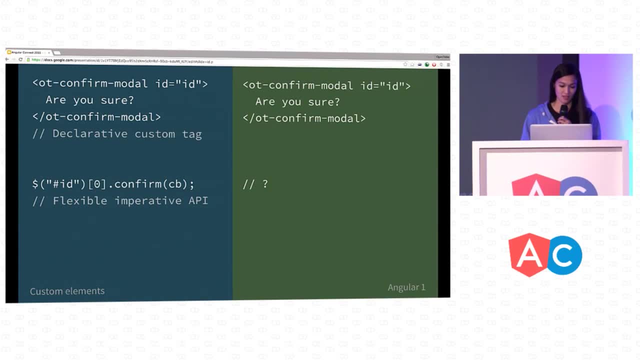 of different ways. The question is: can we create a similar experience using Angular 1?? Let's compare our two features for custom elements. In Angular, you can also add custom tags to the DOM through directives. However, it isn't quite that simple to get a hold of another directive's public methods. 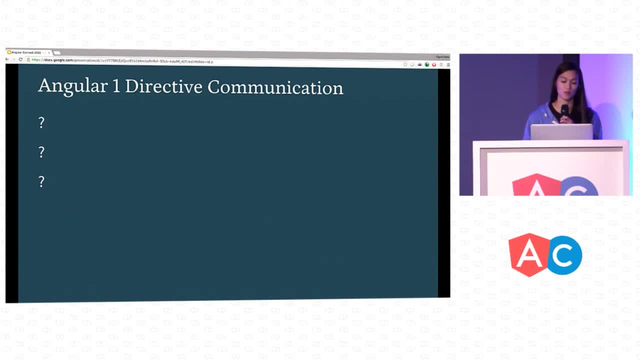 We can't just query the DOM. So if we want to communicate, what are our options? Given the robustness of Angular 1, there are actually a myriad of ways we can approach component communication, Some more recommended than others. In this section we'll use the confirmation model as a jumping off point to explore the 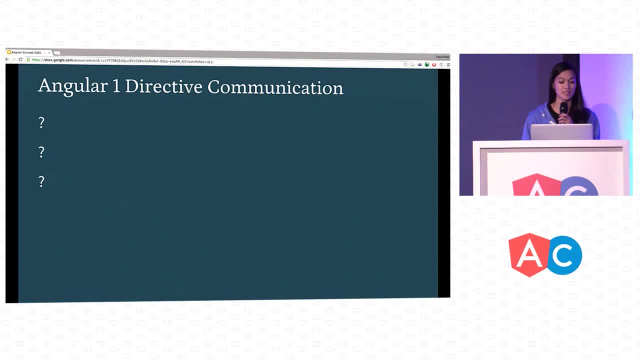 pros and cons of three popular strategies, both from implementation and programmatic interface perspectives. Then we'll actually build the model in Angular 2 to demonstrate how some of its new features can improve our code. So we'll be running through the slides fairly quickly due to time, but it's worth noting. 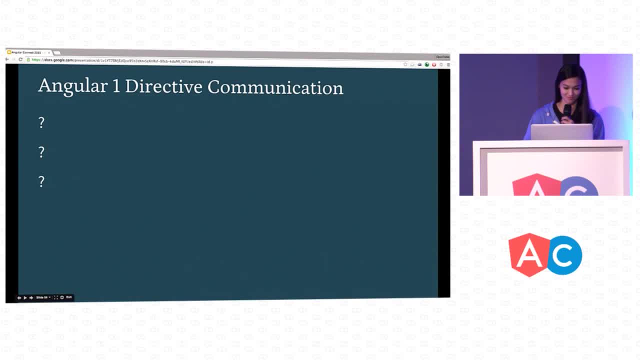 that the again that the full code demos are available online. The first component communication strategy we'll view is an event-based approach. Returning to our confirmation model example, let's say we had a button that did something like blocking reservations once again, but we wanted it to trigger the confirmation model. 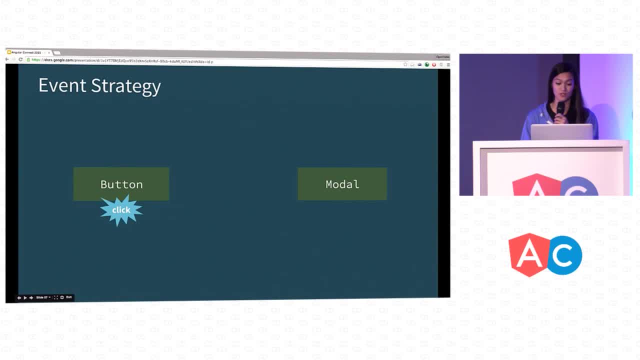 before proceeding With an event-based approach. when the button is clicked, the application might publish a confirmation event and pass through its callback to run on confirmation as its event data. The model would listen for this event and, once one is received, open itself. 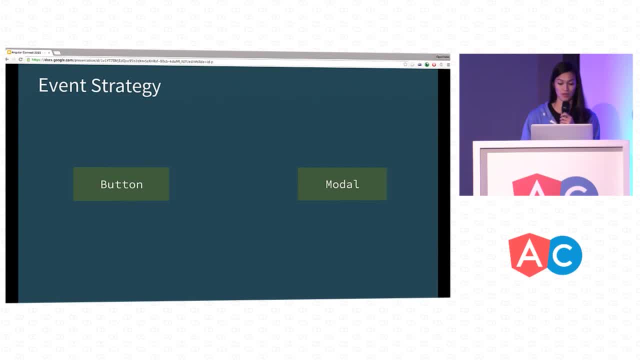 The application could publish the event directly on click Or we could wrap the event logic in an optional trigger directive on the button. Let's say we prefer a trigger directive. So how might we implement this? In Angular 1, you can publish events directionally through the scope tree. 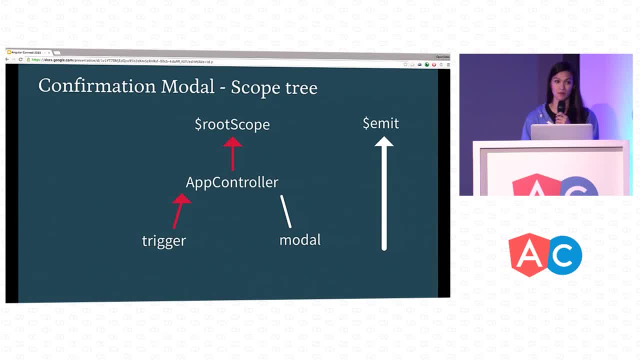 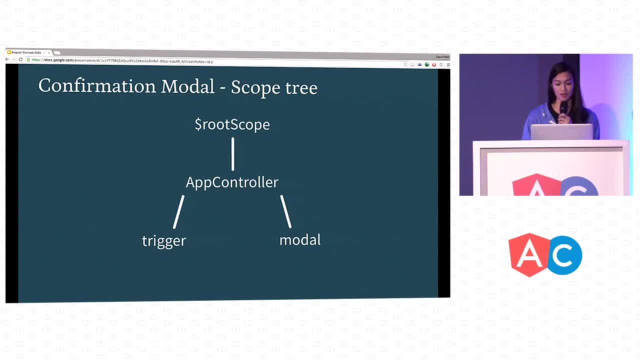 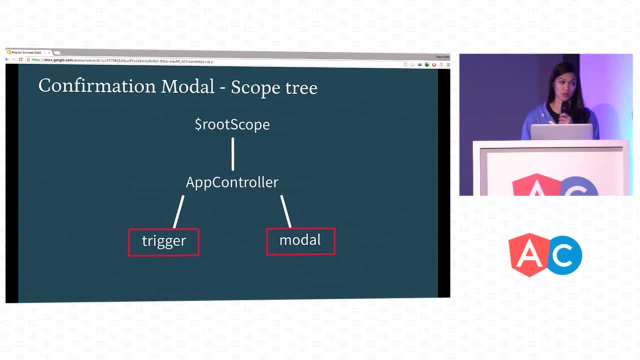 event system. In this case, they happen to both be children of the controller. As sibling scopes, they're pretty much in the worst position because they can't have any direct relationship where one can broadcast down or emit up to the other, Given that our only choice to connect them is to use our trigger scope to emit up to. 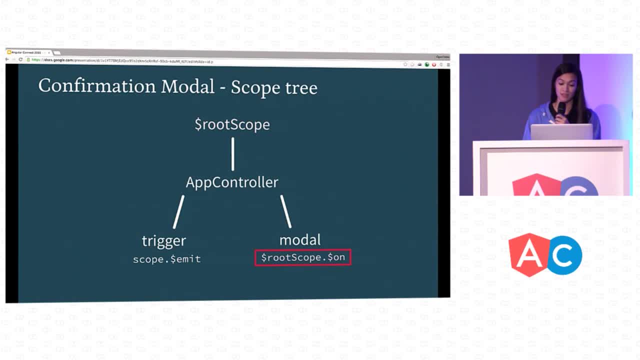 a shared ancestor, the root scope. The modal can then inject the root scope and listen for the event through the app controller. We're going to be able to do that in a couple of different ways. The only choice to connect them is to use our trigger scope to emit up to a shared ancestor. 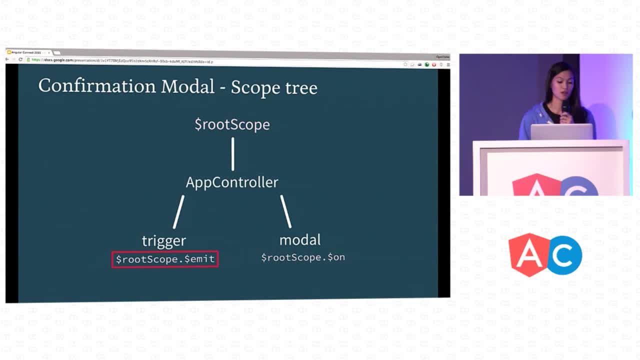 the root scope. The modal can then inject the root scope and listen for the event through the app controller. Given that the trigger can also inject the root scope, we can optimize this a bit by emitting on the root scope directly rather than from its own scope. 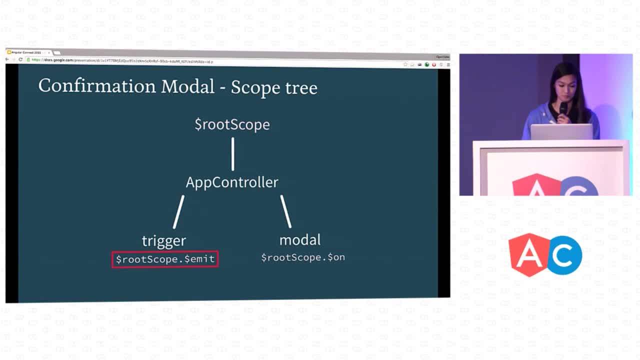 That way the event is only emitted on one level and doesn't have to travel up the chain. And as everything is on one scope, we have to remember to name space the confirm event. so one confirm event doesn't open multiple modals on the page. 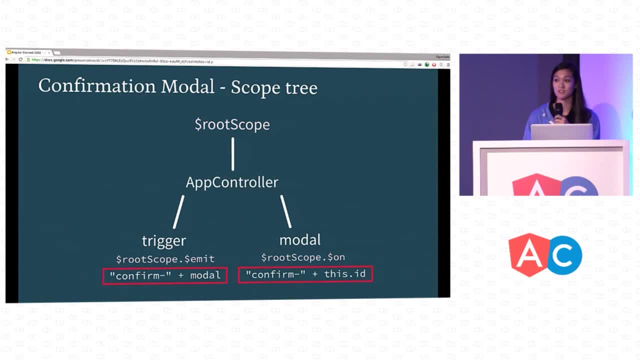 Okay, So let's take a step back. To get this to work, we have to pollute the root scope of the application. This violates the isolation. Even with name spacing, we could potentially run into name conflicts within the app and cause unintended side effects. 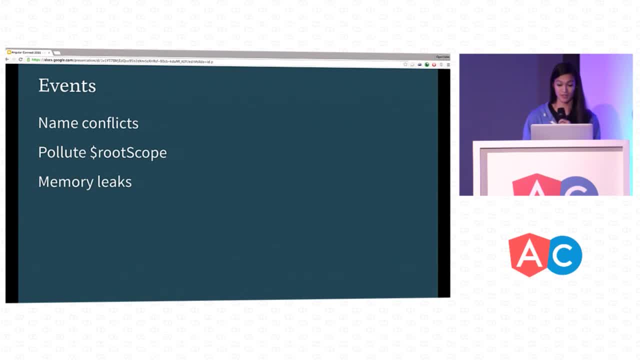 By using global events, we're conducting what should be a private conversation publicly. That's not even mentioning potential memory leaks, if you forget to clean up a listener, which wouldn't produce an error. So the implementation clearly has some drawbacks, but let's check out the flip side of the coin. 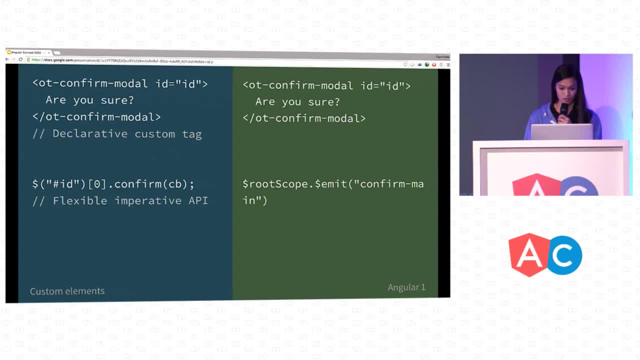 the programmatic interface the events allow us to present. We'll analyze the interface by comparing it to our site. We'll analyze the interface by comparing it to our site. But on the one hand, we did successfully create a declarative tag for the modal. 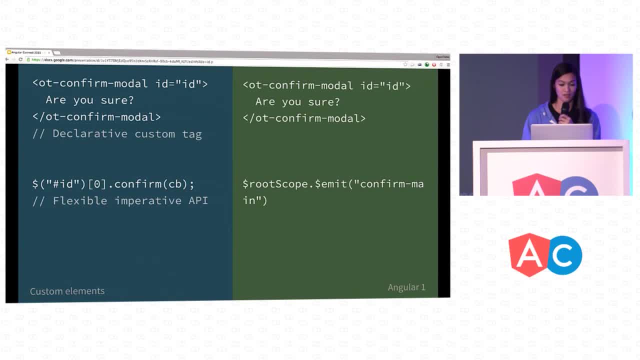 We also provided a flexible API such that it's technically possible to interact with the modal imperatively from anywhere in our application code. The application can choose to emit the event itself Or, if we wanted to, we could add a declarative option for the user, a trigger directive that. 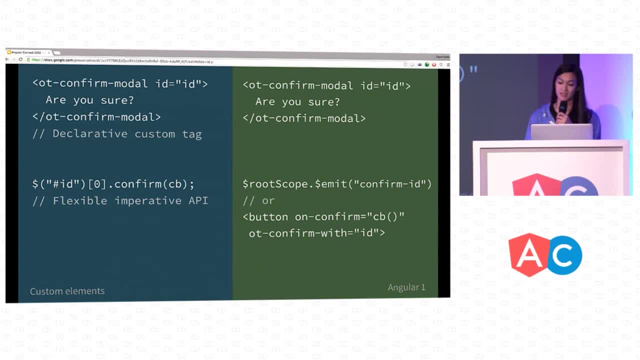 wraps the event logic. It just needs to accept the callback and the ID of the desired modal. From purely an interface level, we're doing okay. But we have a flexible way to communicate with the modal in our JavaScript and the declarative option is quite expressive. We can immediately scan it and intuit how. 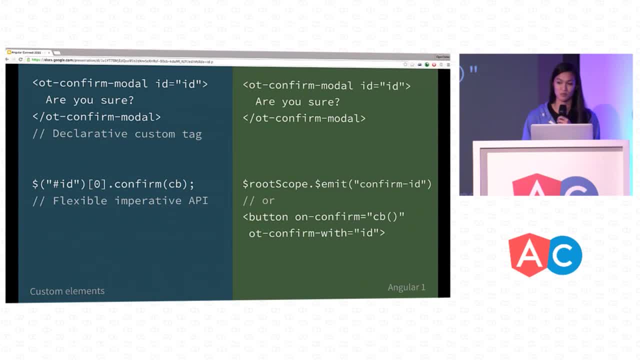 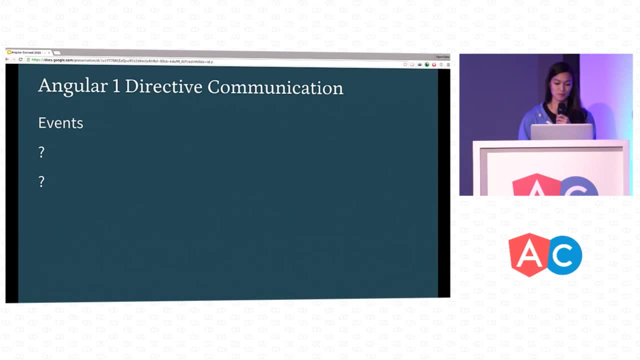 it will interact with the modal, But given that the implementation relies on global events, it's unsuitably risky and isn't a viable solution. We want to find a way to get a hold of the component's public methods directly, without relying on global events. Well, there is a. 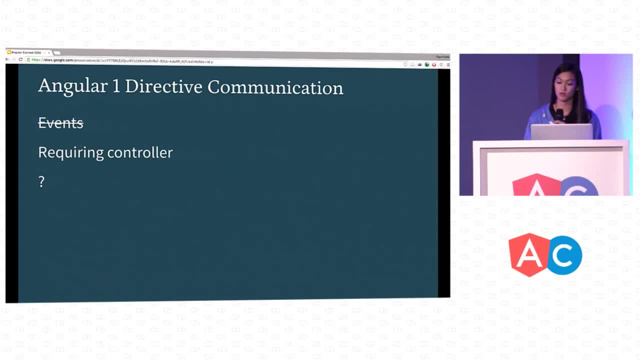 way to do that. The standard way to get the public methods of a component is to require its controller from the directive definition of another component. This simply involves adding the require property and passing in the normalised name of the directive in question. As a result, the controller of that directive will be exposed as the fourth parameter of 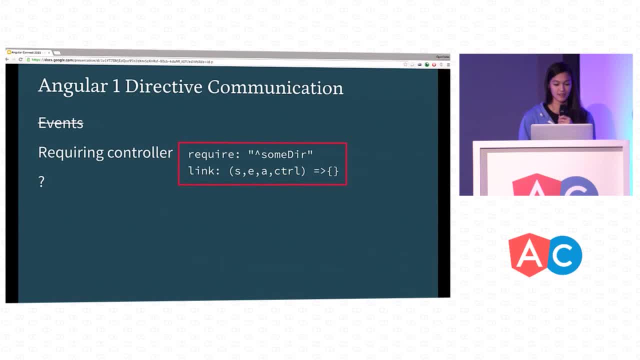 the link function. However, this strategy is pretty limited. Angular can only search for a controller on the current element or an ancestor directive in the DOM. If, again, you wanted the button to open the confirmation modal on click first, you would have to add. 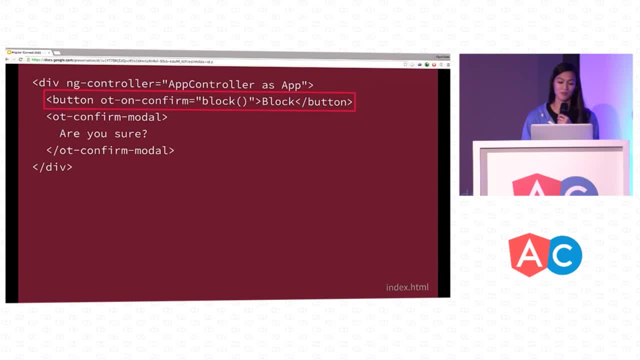 a directive to that button to get access to the require property. and even then it would only be able to get access to the required property and even then it would only be able to look for that controller in its current element, the button, Or a parent directive. 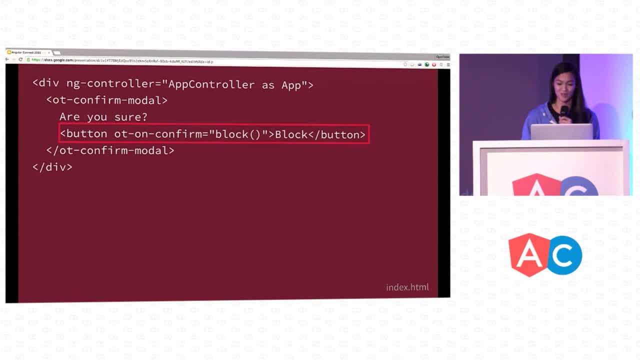 You could try to move the button below the modal on the DOM to make the modal its ancestor, but that wouldn't really work because then the button would be transcluded into the modal. So it's not possible for us to force our two directives into a direct parent-child relationship. 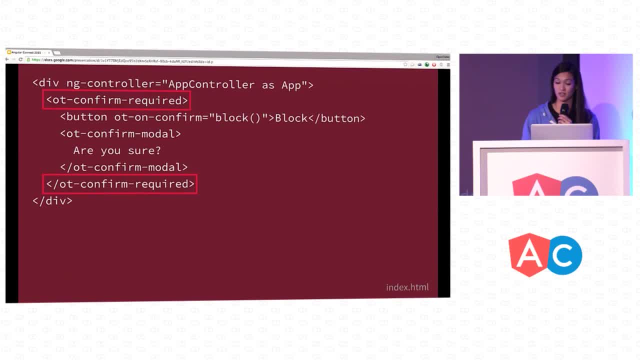 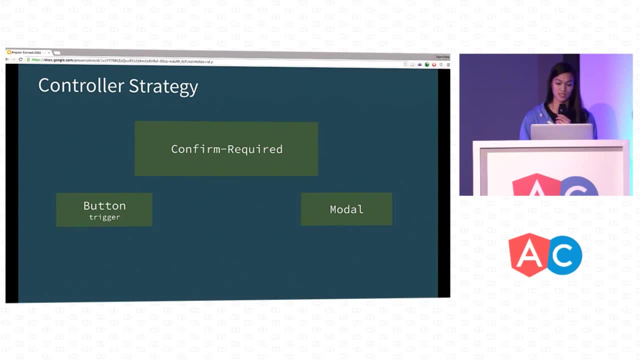 The best we can do is wrap the trigger in the modal in a third shared parent directive so that they both have access to a shared controller. The parent directive would contain all the business logic and state that used to be in the modal and the trigger in the modal would simply pull down that shared logic. This actually 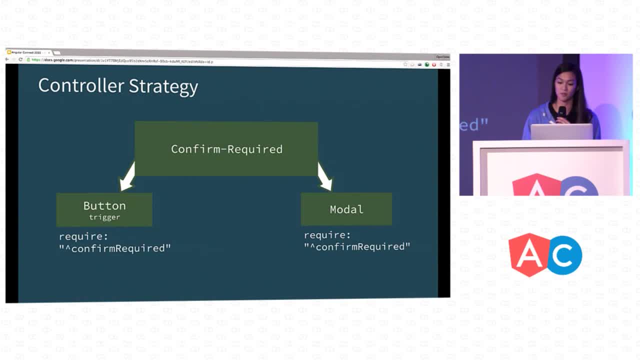 ends up being a simple implementation. All we have to do to connect the button and the modal is push the logic up one level, And in doing so we're not polluting the root scope. So, at least from an implementation standpoint, the controller strategy doesn't. 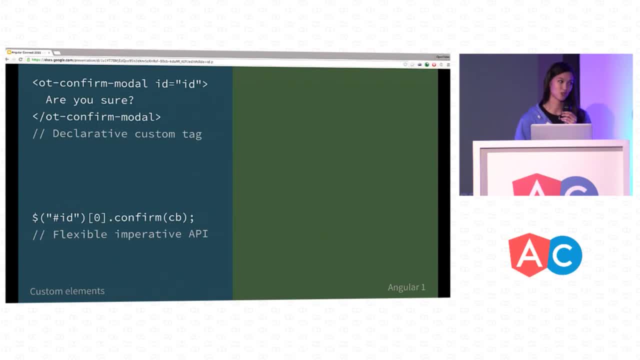 raise any significant red flags. But how does this measure up as a programmatic interface? Again, it's easy to declaratively add a custom tag to the DOM. It's easy to add a custom tag to the DOM, but it's also easy to add a custom tag to the DOM for the modal. And, given that the modal and the trigger 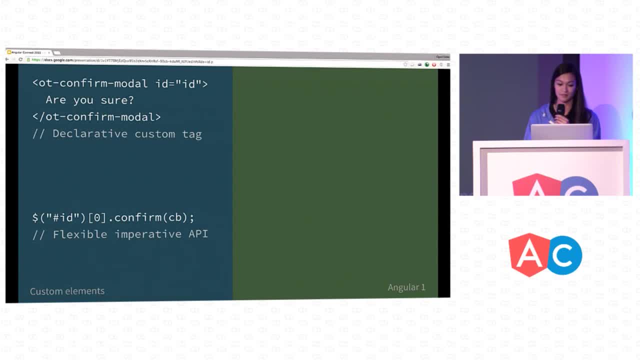 are grouped together under one parent. we don't have to tag either of them with an ID. But this fails the flexibility test Using this strategy. if the application wants to communicate with the modal, there's no way to do it directly from the JavaScript While. 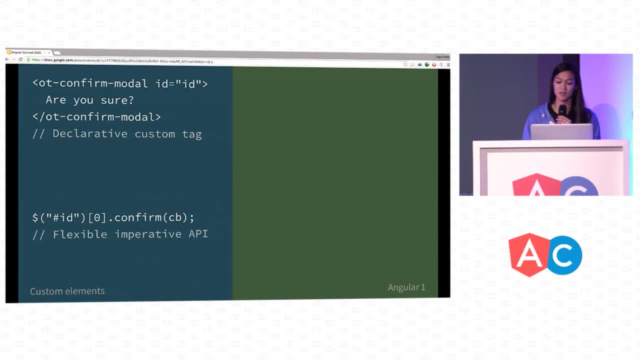 with events. we could choose to create a trigger directive for convenience. in this method, a second directive is mandatory in order to pull down the controller. Worse, it also has to create a third wrapper directive to connect the two directives. This is way too verbose. The problem really is that the controller strategy in Angular 1 has constraints. It was really designed for directives with a parent-child relationship and is a perfectly reasonable approach for those situations. But when you can't guarantee that it kind of falls apart. So again we're running up against the sibling directive problem With. 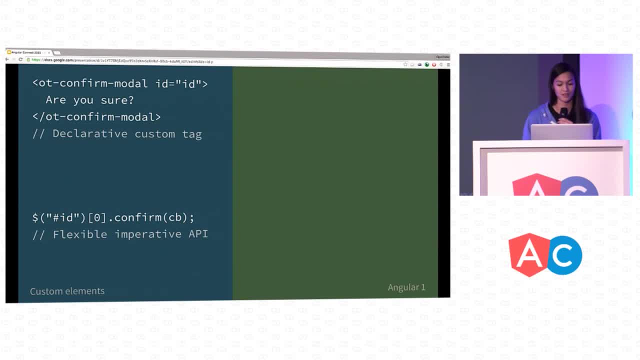 events. the sibling problem lured us to dabble with the dark arts of root scope Here. it forces us into a clunky interface where we have to add three whole events or directives just to get started. Oh, is that not on there? Okay? 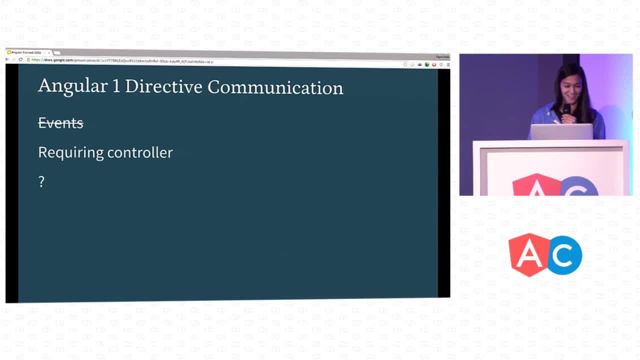 I'm sorry. I'm sorry. Okay, So we want to be able to access the modal's public methods from anywhere in the app without significant risk and without extras like creating a second directive. Well, a service is injectable anywhere, So why don't we just try making our modal a service Rather? 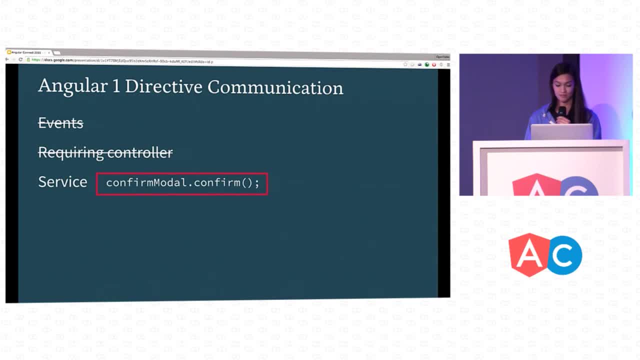 than creating a component we could call confirmModalconfirm directly. How might this work? In the previous approach, the DOM contained two directives that we're trying to communicate Using a service. we don't start with a modal on the DOM at all. 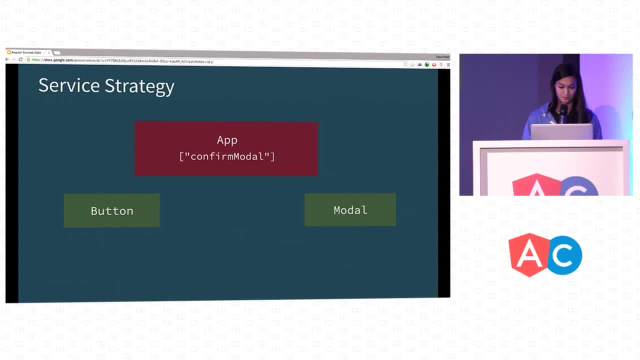 Instead, we create a modal service and inject it into our app. When confirm is called, the service will append the confirmation modal to the DOM, And when close is called, the service will remove the modal from the DOM. The beauty of this technique is that services 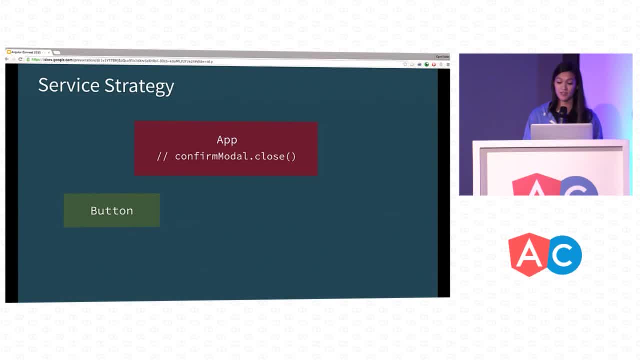 can be injected anywhere we need them. By replacing our two directives with a service, we essentially sidestep the need to communicate between components. Unfortunately, if we don't include the modal directive in our markup, we have to do quite a bit manually to get. 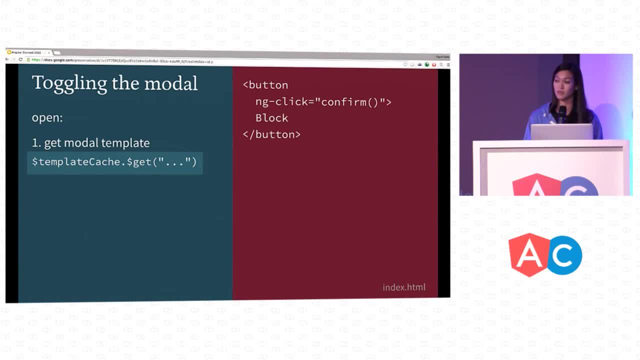 to open it We have to get the modal template somehow, which we can do with HTTP or template cache. And, of course, if the modal isn't in the DOM initially, Angular won't compile it for us. It will only compile what it sees the button, So we'll need to inject the compile. 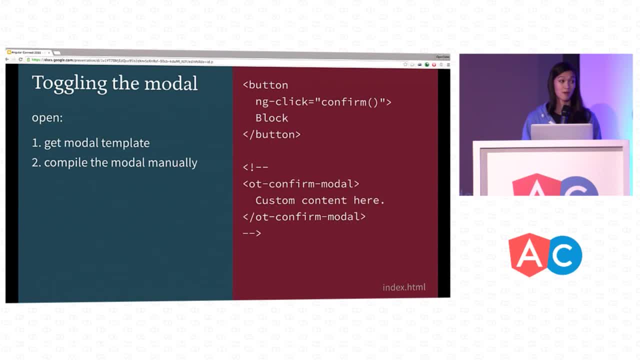 service and do it ourselves. We also have to think about custom content. Previously the user passed content into the modal through transclusion, like on the right, But now our only entry point is its confirm method. So we'll have to pass in a template URL in addition. 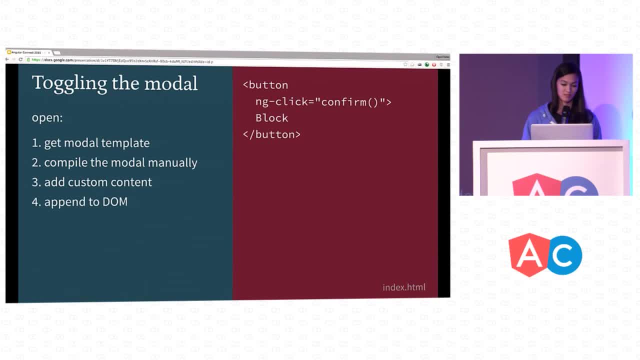 to that. Then we can get the template, compile it and append it ourselves. Lastly, we need to append the whole thing to the DOM. On close, we simply remove the element and destroy the scope. The service approach is convenient to use because it's injectable anywhere, but 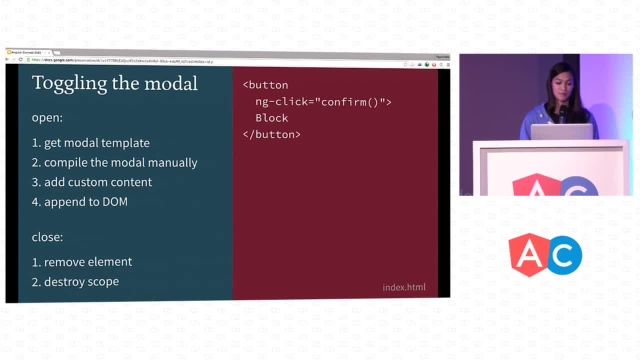 not disruptive to the rest of the app. However, it's a much more complex implementation than the previous two strategies and requires a number of low-level Angular services to work. It's worth considering that this might be a steeper learning curve for new maintainers. 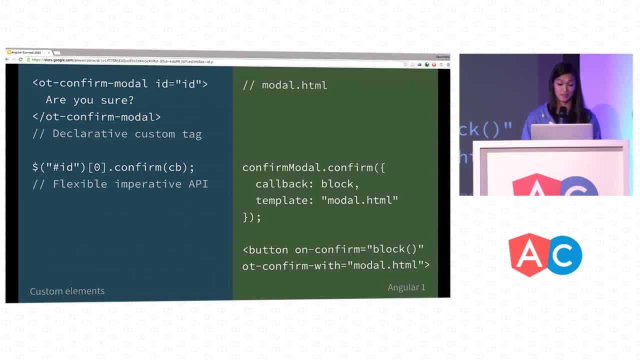 But the real test once again is to compare the developer workflow to custom elements First. it definitely passes the flexibility test. The service provides us easy access to the modals API from anywhere in the application. We simply inject the service and use what. 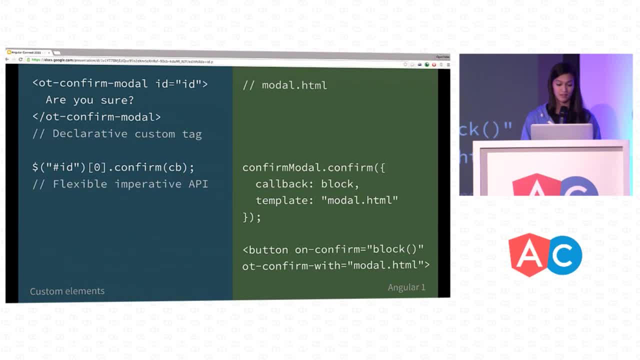 we want imperatively. We can either make the service call directly in the application or we can wrap it in a trigger directive to support a declarative option. All the directive needs to work is the callback and the modal template which it can pass to the modal services. 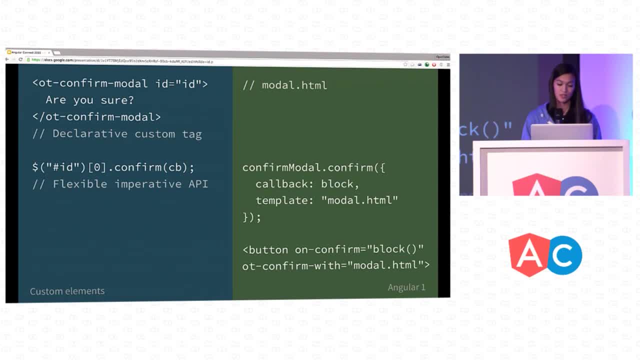 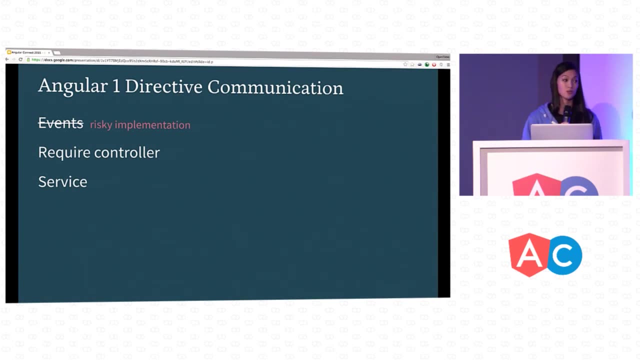 confirm method. The trigger directive option is sufficiently expressive, should we choose to use it. Anyone looking at a button can see that it will open a modal To summarize the event. strategy passed both interface tests, but the implementation was too risky for real use. The controller method works best on parent-child directives, so 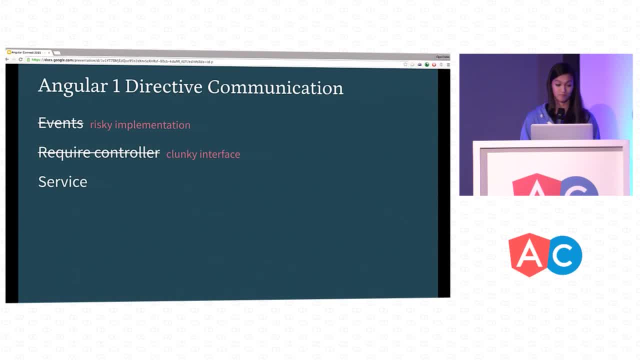 it proved too clunky. Of the three, that leaves us with the service option In Angular 1, we do have to make some compromises. With the help of Angular 2, we're able to get any closer to the custom elements paradigm we've been shooting for, Absolutely Angular. 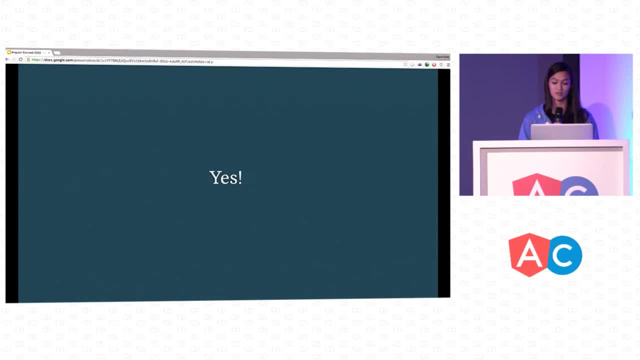 2 provides a host of powerful new features that facilitate building flexible and user friendly component interfaces. In this section we'll build a confirmation model from scratch, using Angular 2, to demonstrate how it's possible to leverage some of these new features. Every Angular 2 component consists of two parts. First we have the component class, which 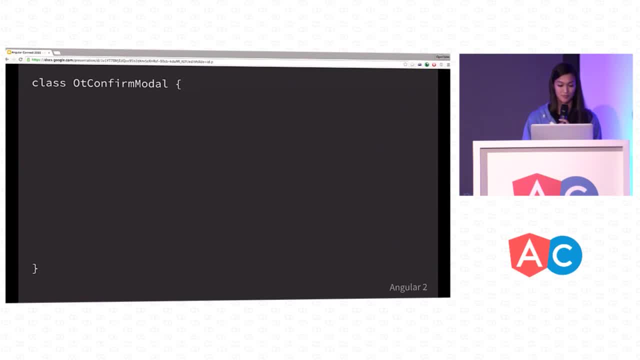 is simply an ES6 class with all of the component's public methods and properties. The second component is the public method. The second component is the public method, which is the public method. The second component is the public method, which is the public method, which. 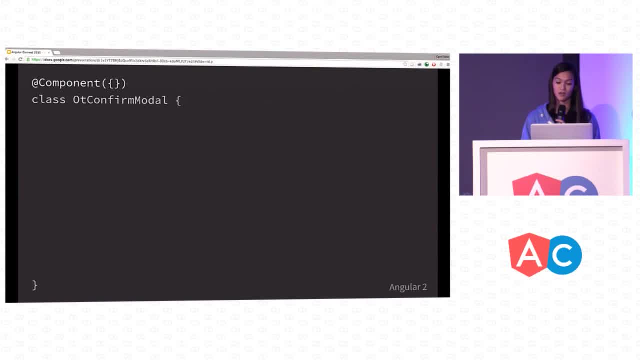 is the public method and the second component is the public method. The second component is the part is its annotations. We can use a component decorator to let Angular know that this class should be instantiated as a component and to pass the configuration options that used. 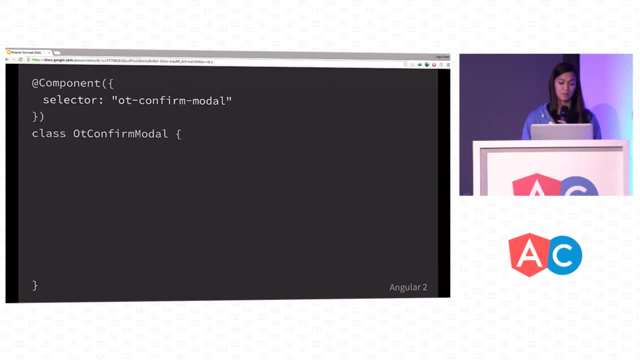 to live in the directive definition, The first of which being the name of the directive, which is now an explicit CSS selector. Next, let's add a template. It's very similar to the one from the custom element section, but you'll notice that we're using ng-content tags and. 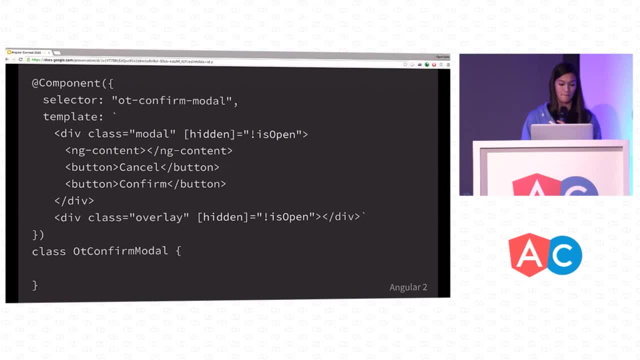 our display logic is slightly different. We're also manipulating the hidden property like custom elements, but through Angular 2's new property binding syntax. We use square brackets to bind the is open expression to the hidden property. It will hide the modal when is open is false. So what's next? We also want to close the modal on click You'll. 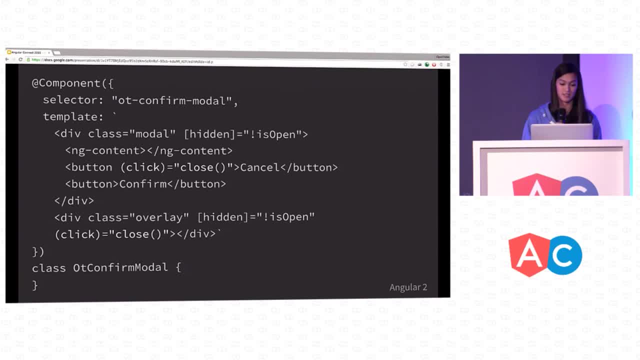 notice that the ng prefix has been replaced by the new event syntax parentheses. Lastly, when the user clicks confirm, we want to proceed to the next step. We want to close the modal and proceed with whatever callback that the user passed in. The template implies three. 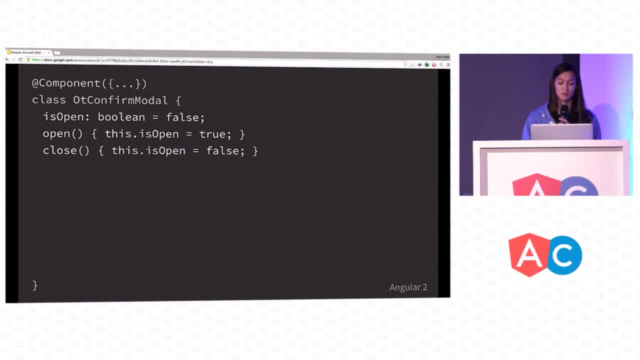 methods: Open, close and proceed. Open and close: simply toggle the is open property And we'll add the same proceed and confirm methods as in the custom element section. To use our modal and to illustrate how it's going to work, we need to create an app component. 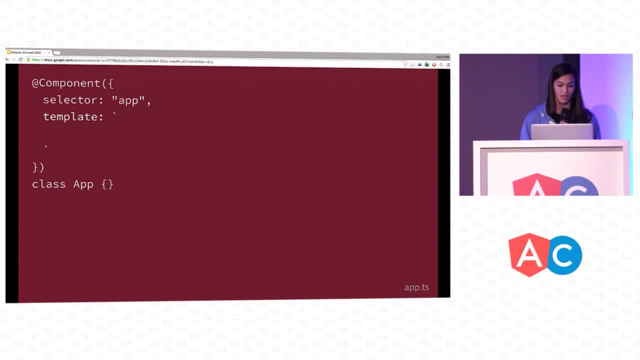 It's constructed similarly, with a class and an annotation, And inside its template we can add the button and the confirm modal tags. Also, we have to remember to add any directives we use to the directives array. So how do we connect the modal to the button? A simple way is to use local variables. Local variables. 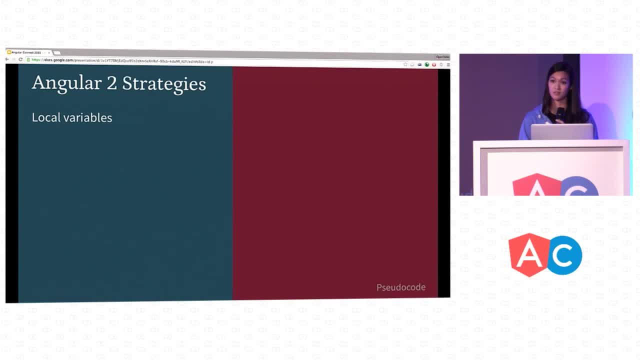 are essentially element or component references that you can create and pass around in your view. You can create one by adding a var prefix or a hash. So adding hash to an input allows you to hook into its properties and print out its value When you put a local variable. 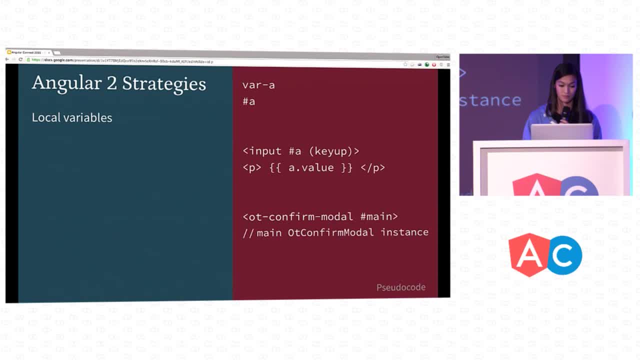 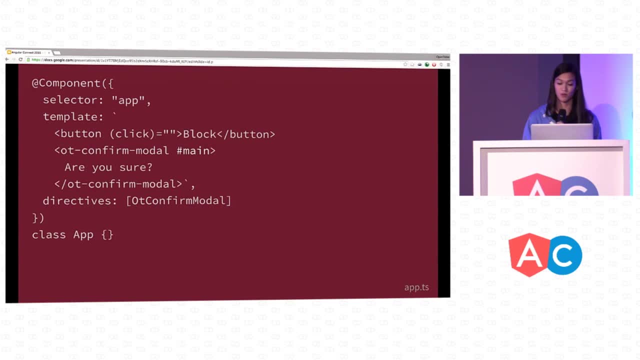 on an Angular component, it will show up as a hash. You can also put it in a part of the. It refers to the instance of the component. So if we add a main variable to our modal, it creates a view variable that maps to the. 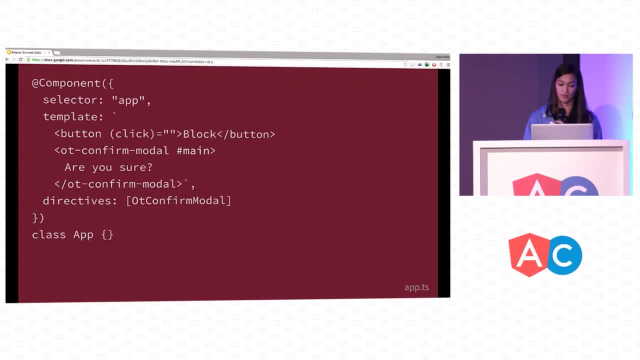 modal instance. This makes the modal's public methods accessible anywhere in the view. This means we can call the modal's confirm method from here directly, So the only thing left to make it work is to fix the context. Currently, any this references in block will point to the modal and not the app where it. 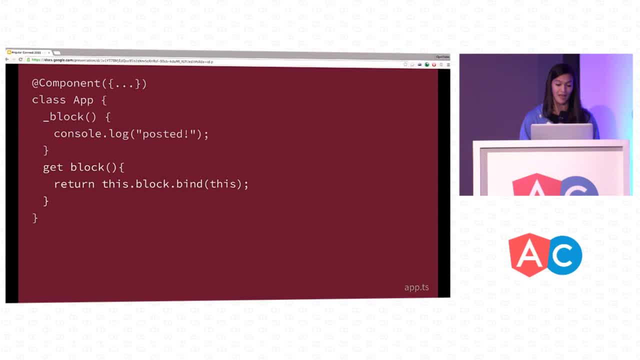 actually lives. That's easily fixable By adding a getter for the method that always returns a context-bound version of itself. While simple to use, this technique with local variables is incredibly powerful and flexible. Any component has direct access to the public API of another component through the view. 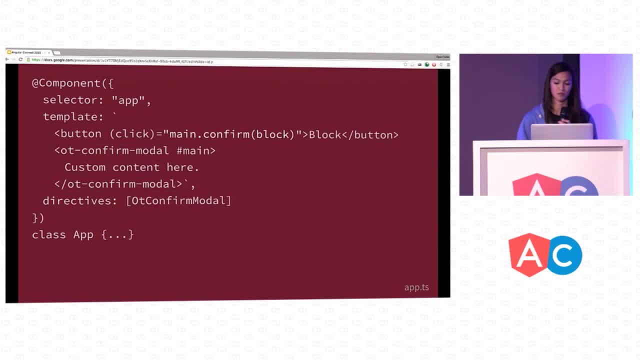 You'll notice that the modal and the button are still sibling elements like before, But we no longer have to worry about that Through local variables. Angular 2 solves one of the hardest problems in Angular 1 component communication. If we change that. 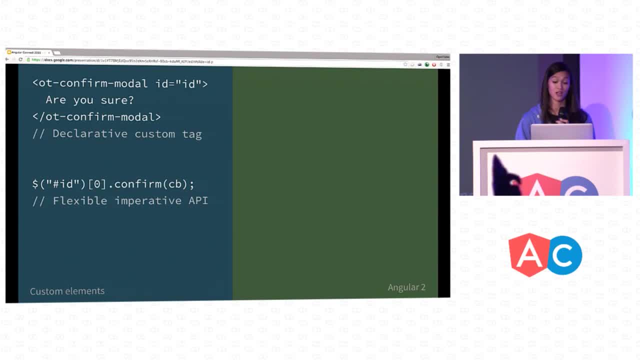 If we take a look at our interface already, you can see that Angular 2 has done a phenomenal job mimicking web standards. It's almost the same. We have the custom tag and we can access the component's public methods from anywhere we like. 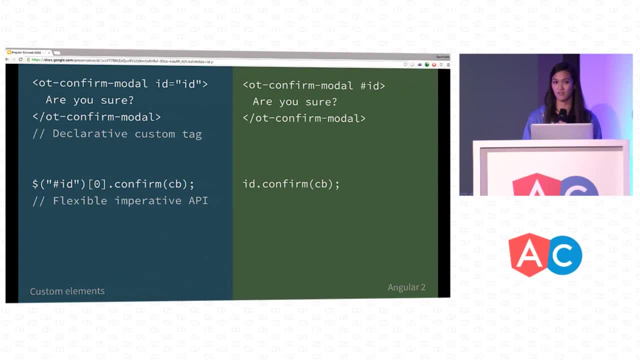 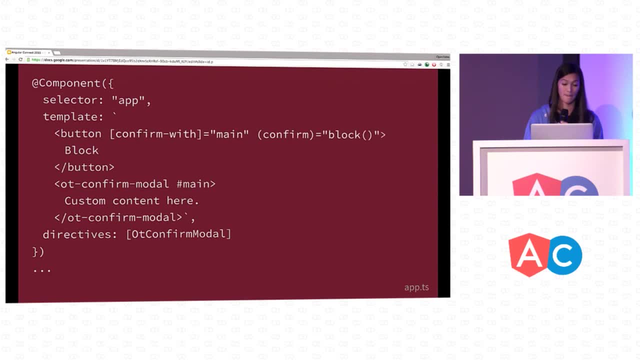 Whereas in Angular 1 we had to accept some tradeoffs, in Angular 2 we get both of the advantages. This also means that we can optionally support a trigger directive if we prefer something that's fully declarative. It's an interesting setup to explore because it's pretty expressive. 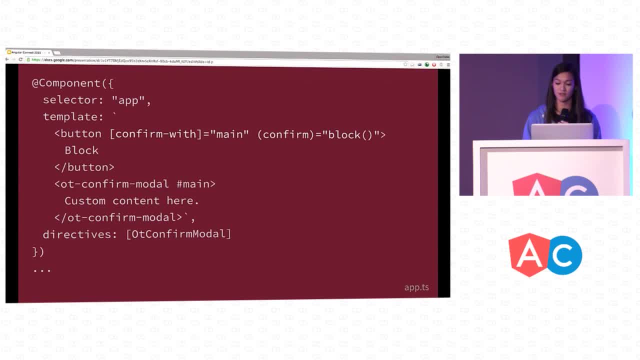 We can immediately tell that we'll want to confirm with the main modal, But, frankly, we'll build this out just so we can play with some more Angular 2.. So how will this work? We're creating an attribute directive called confirm with, and we're directly passing in 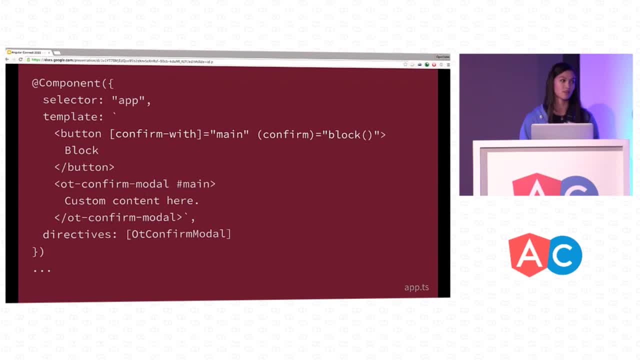 the local variable from before as its input. That's how the directive gets a hold of the modal instance. There are other ways to do that, through querying, which you'll hear about in other talks. But since the modal isn't in the button's view or its content, we can't use that. 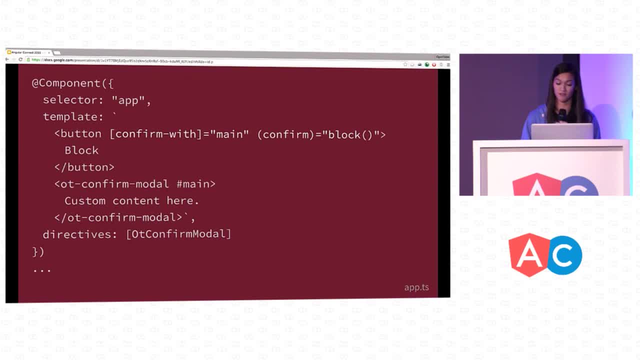 So the second thing we're doing is calling the block method when our directive emits a confirmation event, Which implies we need to create an event emitter. So let's quickly build this, since we're running out of time. Again, we have a class, but this time we're using the directive annotation. 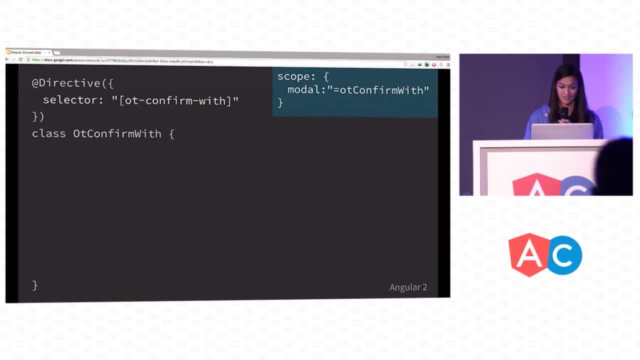 That just means that it's a component without a view We pass in our selector. as it's an attribute directive, it's wrapped in square brackets. Second, we want to support passing in the modal as an input, which previously would have gone to the scope objects. 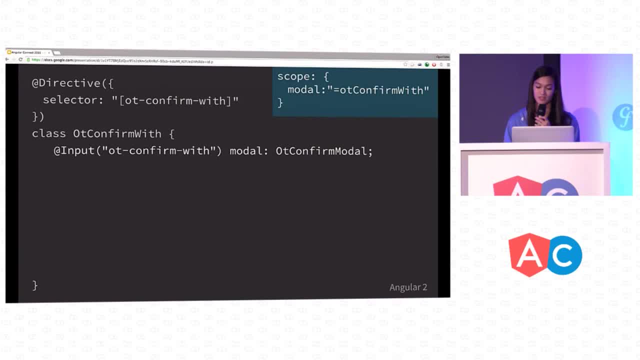 Here we create an input annotation that takes the OT confirm with property and associates it with the modal property. on the class, On click, we want to request that the modal In Angular 1- we might have injected the element and called it that way on top. 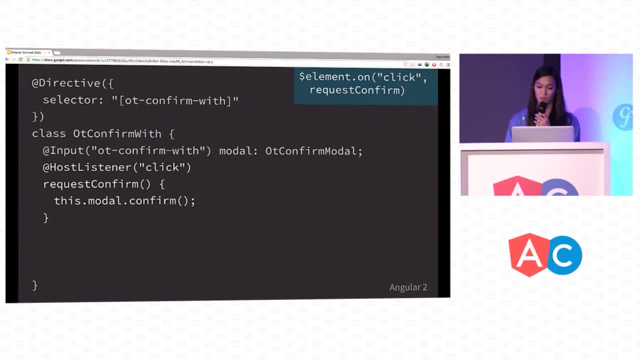 In Angular 2 we can use the host listener decorator with the method it should call, request confirm, And that method will delegate to the confirm method of the modal. Lastly, we want to emit a confirm event from this directive So we can call block reservations, call back. 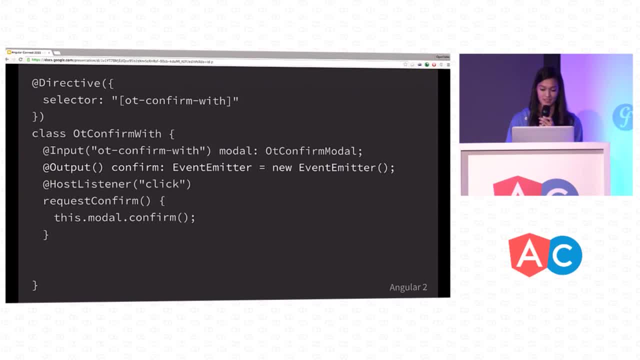 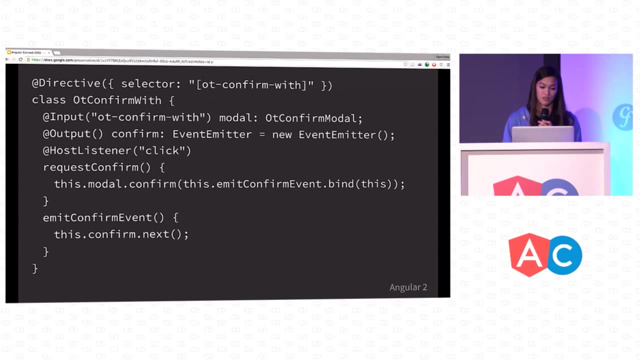 To emit the event. we can add an event emitter class to as thisconfirm and annotate it as one of our outputs. And we can add an emitter And you can pass it in as a callback to our existing modal flow. So that's it. 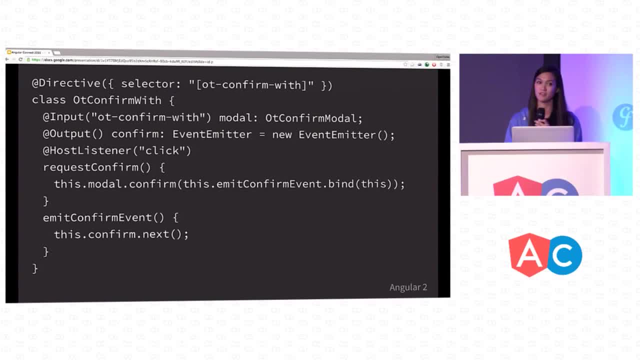 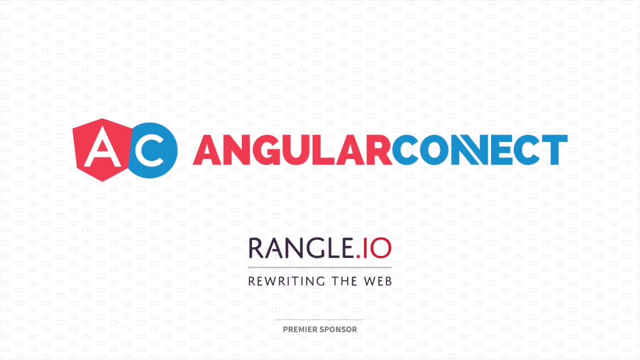